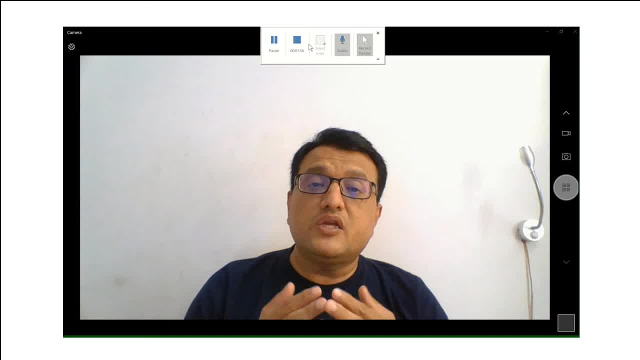 Okay. And also customer also will be having a choice of selection of the suppliers, Like as on: today we are buying a product called a three star, four star for air conditioner, freezes, TVs, et cetera. Everything is having a star rating. Why? Because higher the star. 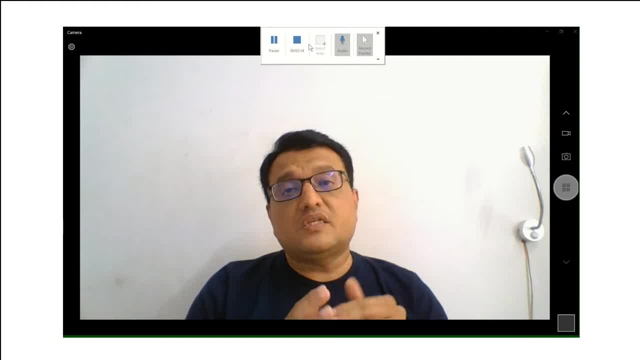 higher the energy efficiency. Similarly, there will be a star for carbon credit also. So it is a right time to understand that. how to calculate the CO2 emission for our own ourselves, as an individual? Also, we are. we are using electricity, We are using cooking. 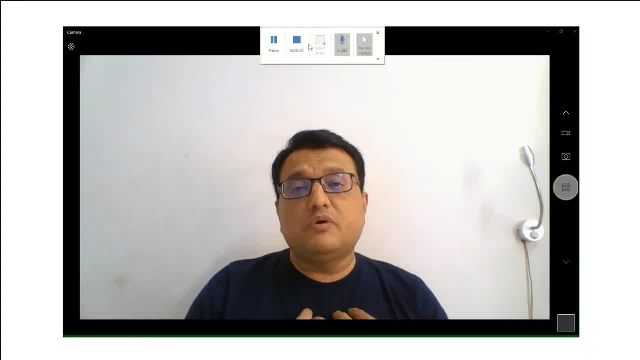 gas. We are driving cars, So we are also responsible for generating CO2.. So I will tell you how to calculate this CO2 emission for any establishment or for our sales, And this calculation is going to be very helpful as far as their academic purpose or for the professional things like. 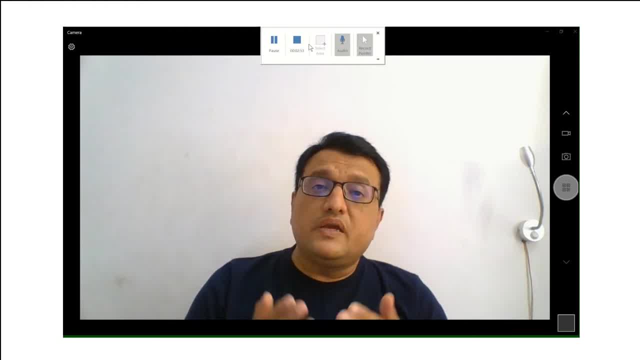 that There are chartered accountants who is keeping record of our, our loss and profits, and all this, and annually they, they publish, they give us a entire books of, you know, balance sheets and everything similarly. such carbon reporting is mandatory and there is a audit called government audit, factory audit, energy audit, sustainability. 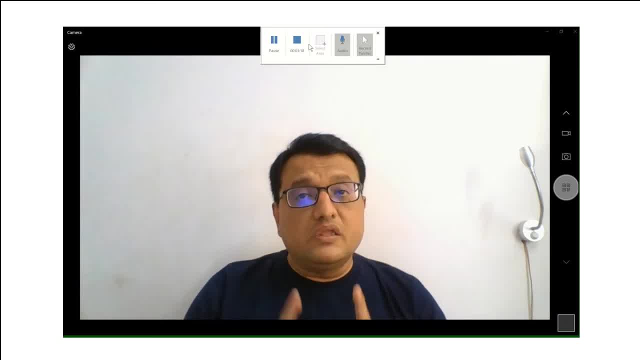 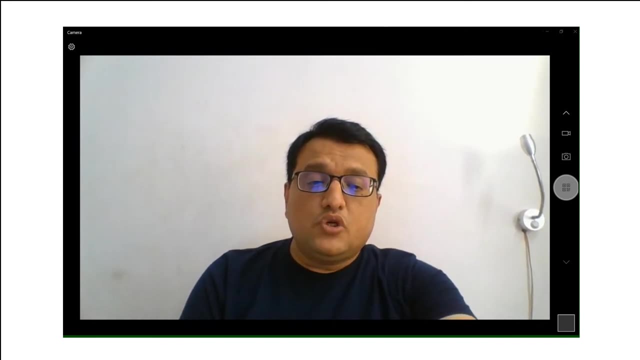 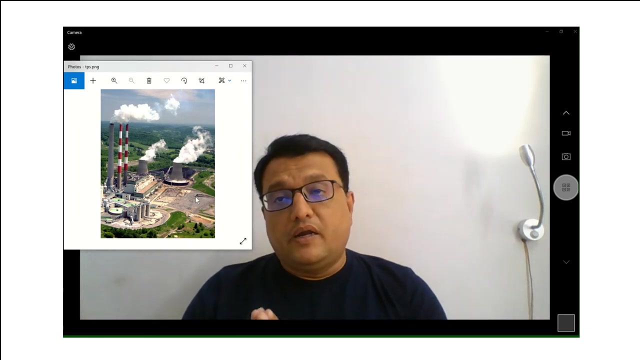 audit, then environmental audit. in all this audit, carbon credit and evaluation of carbon emission is mandatory, and that's why every engineer has to know this calculation. so let us start our thing. i will just show you the one picture here which will tell you that this is the picture which you can see, that this is a thermal power plant. so in india, maximum power. 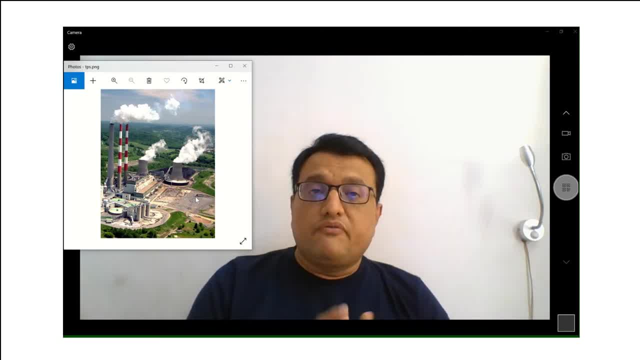 is you know what we are consuming. in our factory or in our houses, in the colleges, in the government offices, in the shops, everywhere, maximum power is coming from the government owned electricity company or privately run electricity company. and this all power plant is running on the coal base. they are using coal to generate the power. 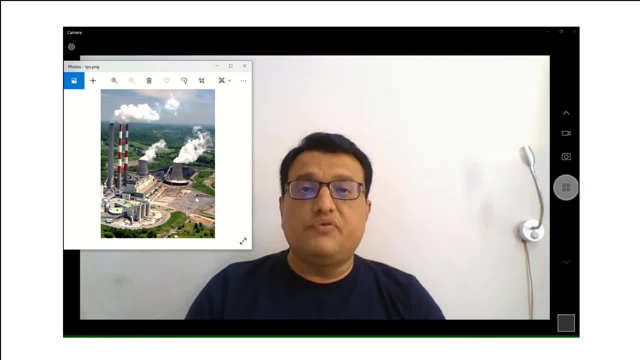 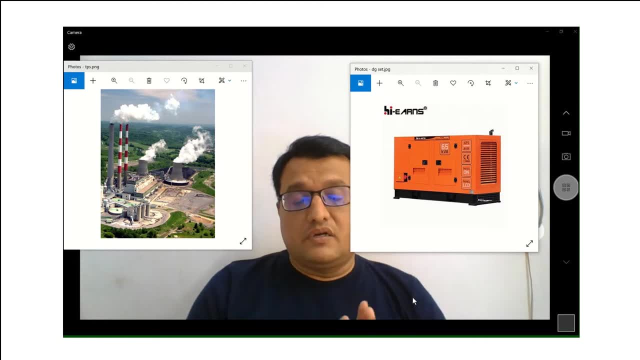 okay, and when this power fails, so we are using a backup power system that we can say it's a generator. so in this picture you see this is a generator. so when the electricity is there from the uh distribution company, that is our first priority is the cheapest electricity, and once this is not available, that time we are using the second source. 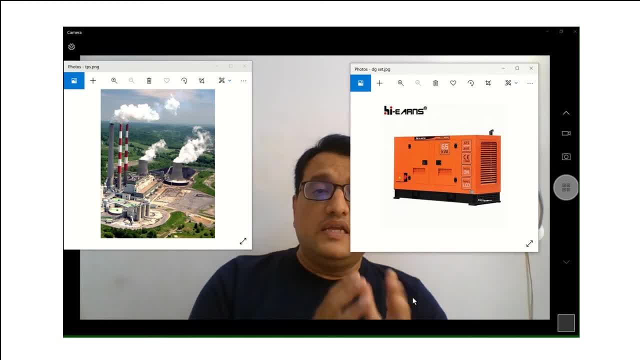 which is we called a diesel generator. and when the diesel generator is running, it uses a diesel as a fuel, so both has a different impact as far as the co2 emission is concerned. so we will calculate the our power. uh, whatever the power we are buying from the electricity company, because that is registered. 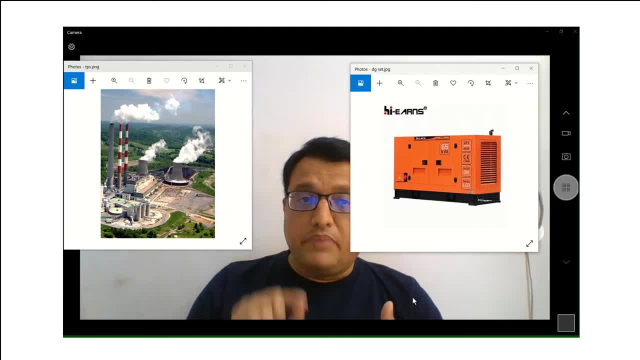 in our electricity meter we are getting into the electricity bill also so that we will take it from there and from there we will calculate- and in the diesel generator said we know that- how much diesel we have consumed in a monthly basis to generate x amount of power, x amount of units. 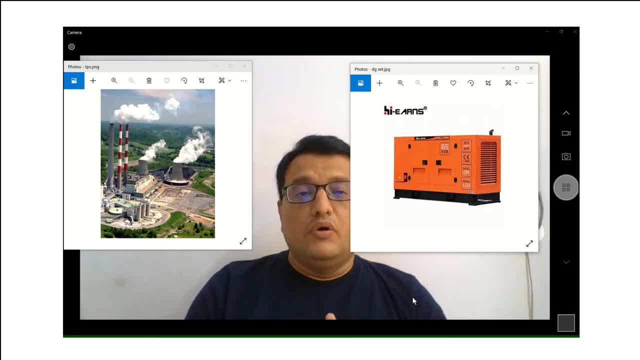 based on the later consume, we will, you know, calculate the co2 emission from the diesel, and then we will combine both together. this is a total co2 emission from electricity as well as the diesel generator, and thus we have to report like this: much of kilogram of co2 or ton of co2 per year we are generating. so let's now i will take you to the 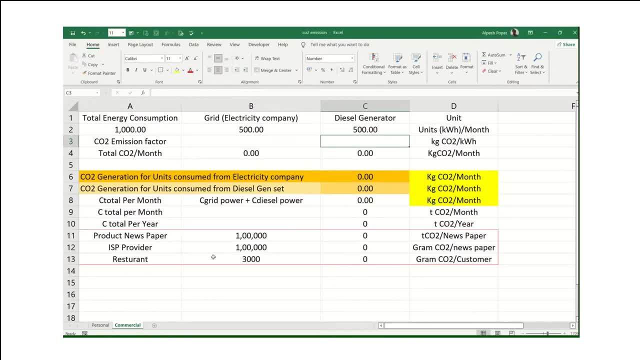 one small access sheet which i have prepared, and here i have created two cases. okay, in the one case, which is a commercial case, like you know, whether it is a factory or anything else, you can just put your whatever your total energy consumption, for example, here i have mentioned thousand units, thousand units per month. unit is there in column. 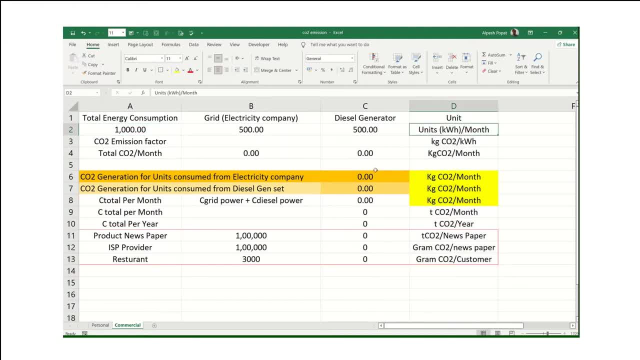 number d here so you can see the units. so thousand units i am consuming per month, in which i have divided my requirement in 50 in the electricity company, which i am taking 500 units from electricity company and rest 500 units i am generating by installing my own diesel generator. 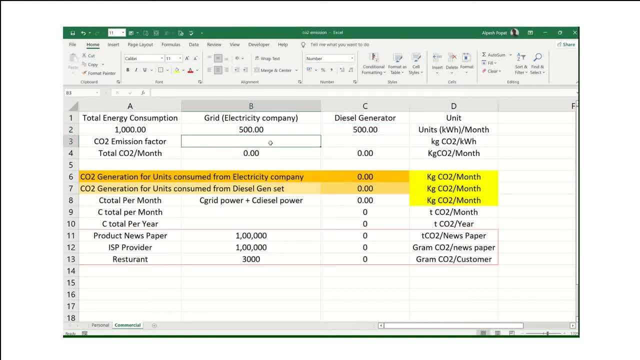 set. so now we need to see that. what is the emission factor? step one is over that we should understand how much electricity we require and out of which, how much we are buying from electricity company and how much we are generating from dg set. second one is emission factor, so i will take you to the 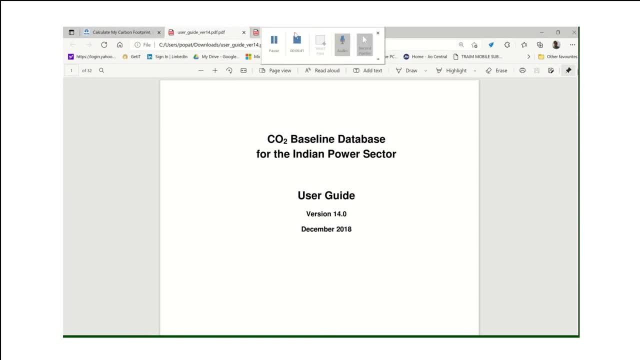 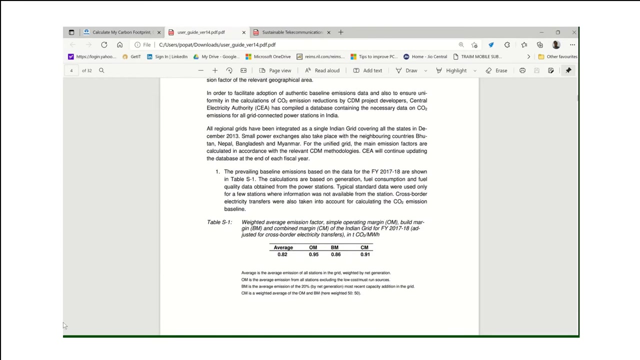 one government guideline is there here, okay, and this guideline tells you that how much of you know here. if you see this, then this is a guideline from the central electrical electricity authority. okay, it's a government of india's body and it is saying that here. if you see, this is a 0.82 kg. okay, let me just enlarge here. 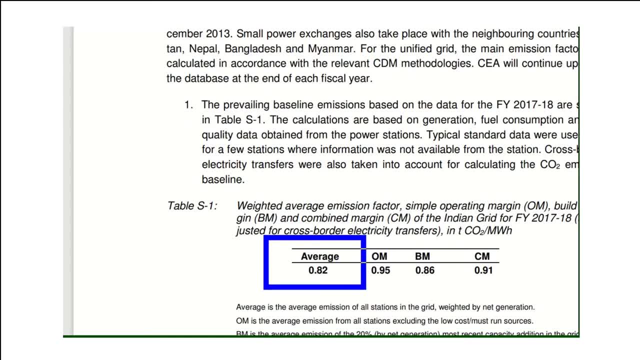 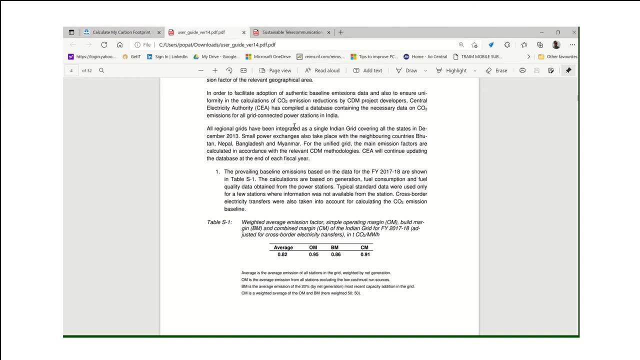 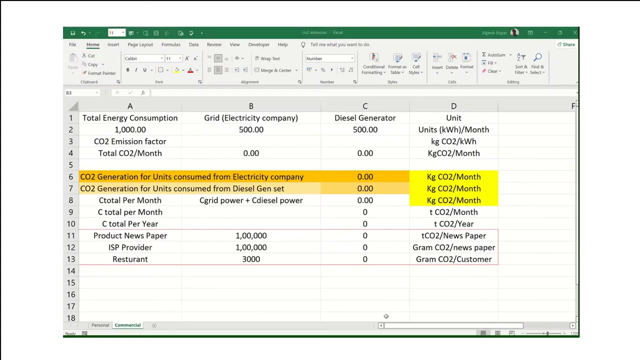 so at least we can understand. this is a 0.82 kg of uh. so in this government guideline emission factor is mentioned, which is a 0.82, right. so this 0.82 kg co2 per 1 kwh, that is what the meaning is. so let us now go to our excel. 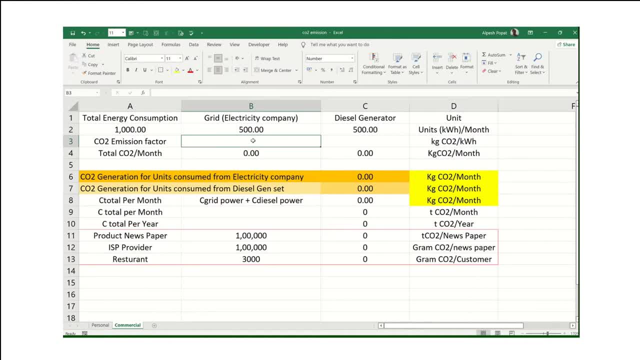 so we are consuming 500 units from the company electricity company and for one unit it is a 0.82 kg co2. so that means 410 kg co2. we are producing uh into the environment per month because our monthly consumption is 500. so this 410 is for this 500 unit consumption, which 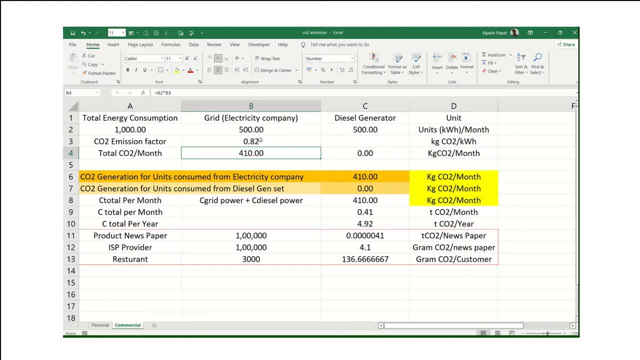 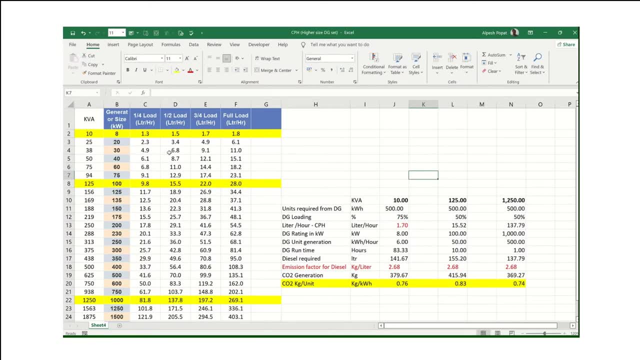 we have taken from the electricity company now. second one is the diesel generator. so for the diesel generator we have made one beautiful sheet which is very helpful here. now dg set is is having a different size of rating, which is starting from 10 kva to 2000 kvm. so every customer has a different rating of dg sets in. 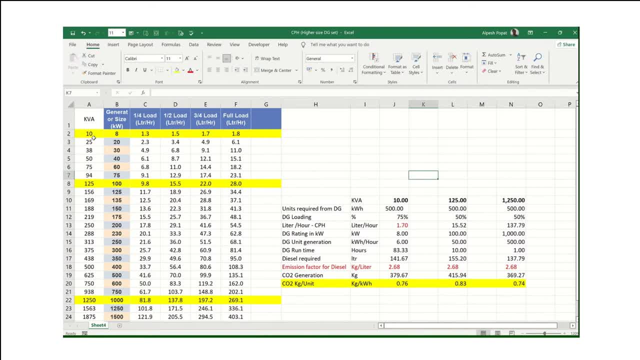 their premises. so that is why i have taken a three different case. one is the very small rating of dg set, another is a medium sized dg set, which is a 125, and another one is a large dg set, which is a 1250 kva dg sets. and we will calculate the same that our reward is, our requirement, our 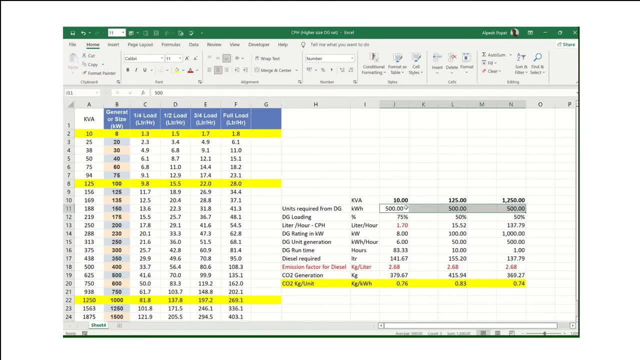 requirement is 500 units. we need to generate balance 500 units from the diesel generator and for that how much diesel will be consumed, and based on the diesel consumed, we will calculate how much co2 will be generated. that is what our objective. so now let us start for the 10 kvm. 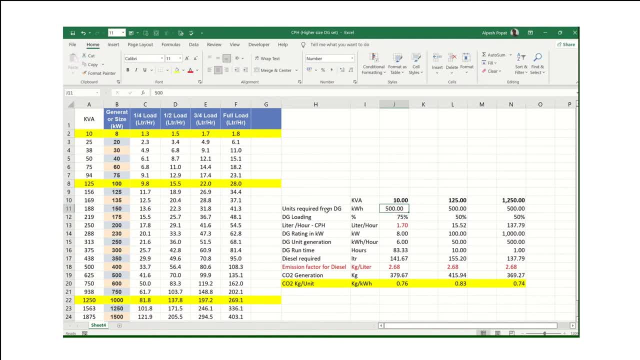 now here, the second row is units required from dg, which is 500 units, and these 500 units kwh is for month, monthly basis. now, what is a dg loading? dg loading that means, if you see, in this chart we have mentioned, is: this is a 75 percent loading, this is a 50 percent loading. 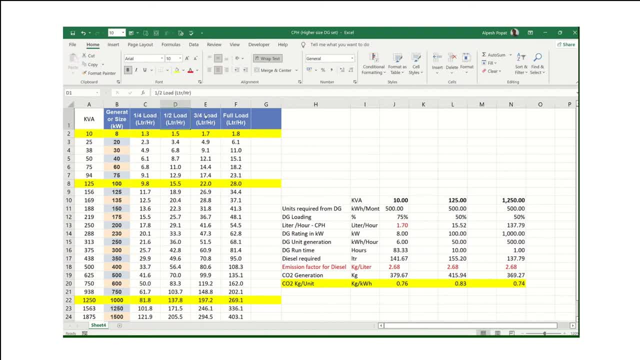 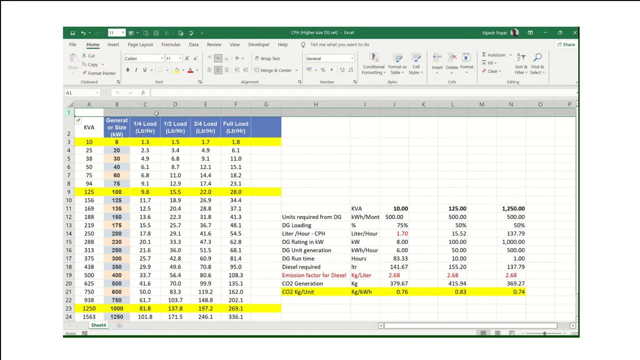 uh, this is sorry. the first one is 25 percent, this is, uh, 50 percent, this is 75 percent and this is a 100 percent. so let me just mention this so it is easy to understand. this is a 25 percent of load. that means, whatever the capacity is there, we are using 25 percent of its. 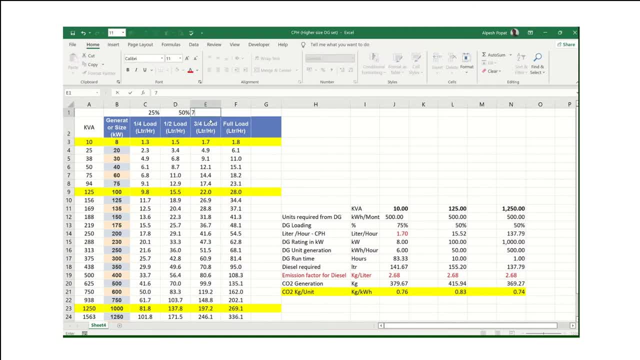 dg capacity here is 50 percent, this is a 75 percent and the last one is 100 percent. so here we are, using us. we are running our diesel generator, which is a 10 kva. we are running on 75 of load. okay, so if we are talking about our fuel cell consumption per hour or our fuel capacity per hour, 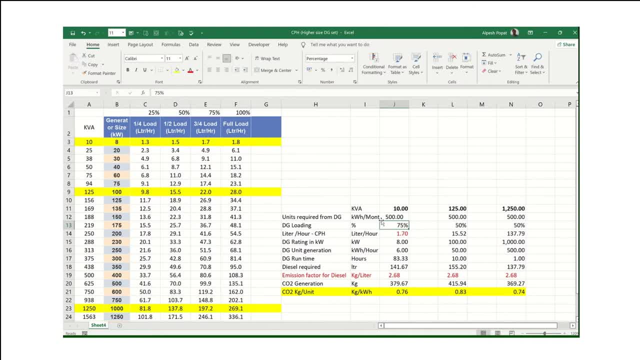 this is your assumption that anybody can uh see their dg set that, what the loading it is running, whether it is running on 50 percent, 100 percent, 25 percent, whatever. now, if my generator is running on, let's say that on 50 percent of uh 75 percent of load which i have. 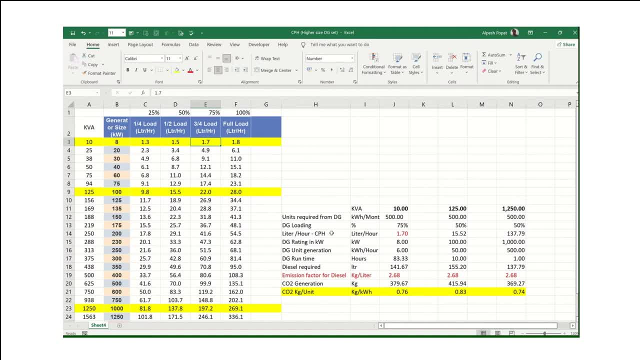 taken here, that means it will consume 1.7 liter per hour. okay, so i have taken what is my cph, that is, a consumption per hour, which is a 1.7 liters per hour. per hour. Now, 10 kV DG, that means it is a kilowatt capacity is 8.. Everybody knows we have to. if you 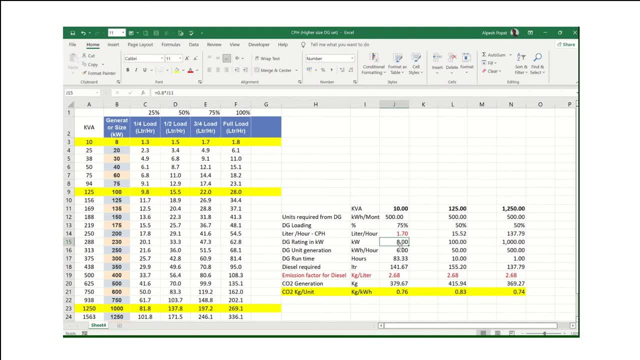 don't know you to multiply this 10 into 0.8.. So you will get 8 kilowatt. So technically, 8 kilowatt is the final rating ultimate capacity of the DG set. Now we are not running ultimate. that means. 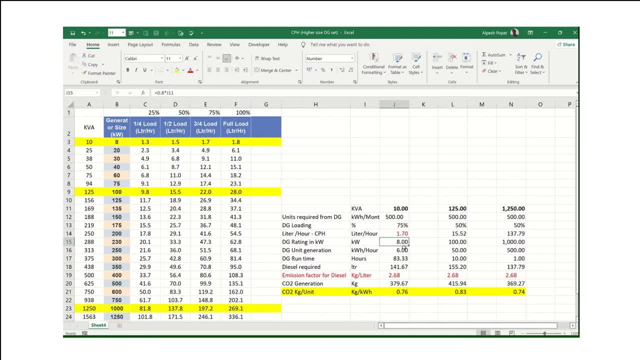 100%. We are running our DG set on 75%. So when you multiply this 75 into 8, that means you will get your 6 kilowatt of load. What is the meaning of this? My 8 kilowatt of diesel generator is. 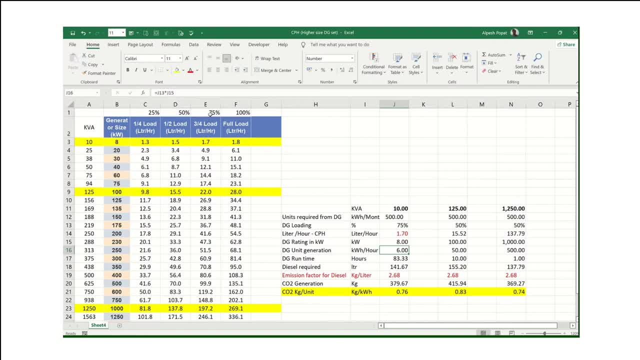 running on 6 kilowatt of load, which is a 75%. So when my generator will run one hour, it will produce 6 unit. Okay, So how much unit I want to produce? So this is already. I have mentioned that I want to produce a 500 units, right? So what I will do? I will divide 500, divided by 6.. So I will get 83.33 hours. That means my diesel generator has to run 83.33 hours to generate 500 units, And when DG will run for 83 hours, every hour it will consume 1.7 liter. So for 83 hours. 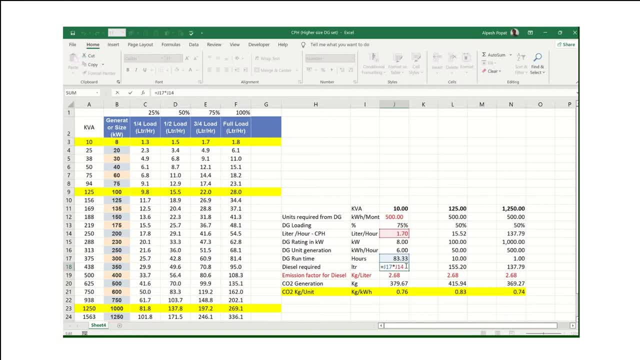 if you see here, it will consume 83.33 into 1.7, which is equal to 141.67 liter of diesel. So this amount of diesel is required in a month. okay, to generate 500 units. Now there is a emission factor. for diesel generator, which is a 2.68 kg. That means when 1 liter of diesel is burnt, 2.68 kg carbon dioxide is emitted. So we need to multiply this 2.68 into 141 liter, So we will get 379.7. 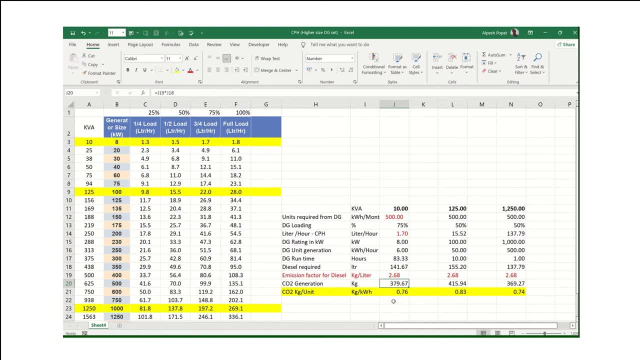 six, seven kg of co2. so now, if I want to calculate what is a per unit generation, because I am, I have consumed, I am- I am generating 379 kg for 500 units. so for one unit that means three seventy nine point six, two divided by 500, which is nothing but 0.76 kg per one unit of DG set. okay, now let us see on the one more capacity of the DG. same way, if I am putting 125- and I am assuming here that my 125 kVA machine will run on 50% of load, that means at 50% it will consume. 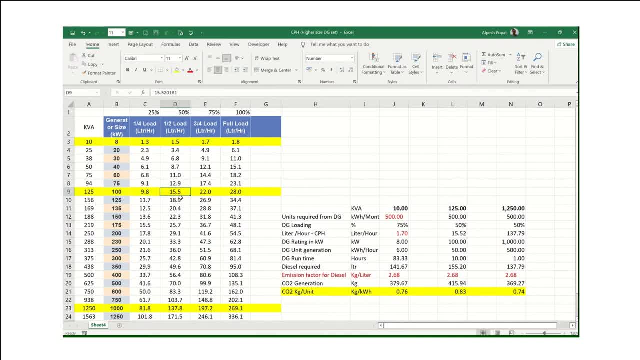 15.5 liter for one hour of running. so I have taken 15.5 and DG rating is 125. so when you want to convert this 125 into kilowatt, you have to multiply 0.8 here. here also mentioned 125 kV DG is equal to 100 kilowatt. okay. 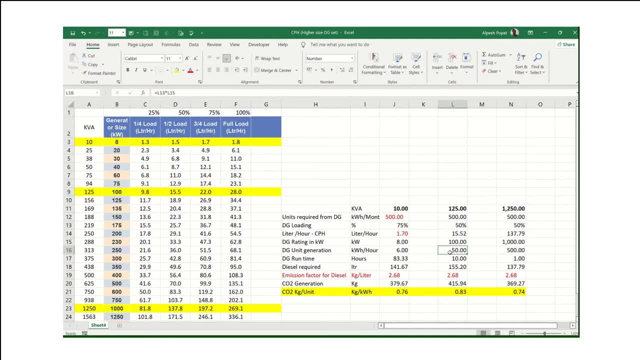 and one. once my DG will run for one hour, how much it will produce? because it is running on 50% load, so 50% into hundred, that is 50. so one DG will run for one hour. it will produce 50 units. how much I want to generate? 500, so I will. 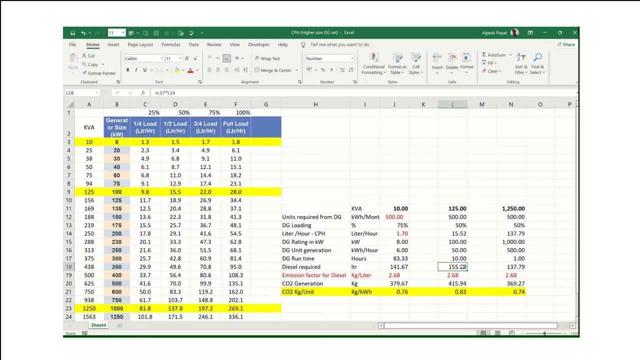 150, 5.2 liter of diesel is required to generate 500 units. okay, and our emission factor is same. that 1 litre is is generating 2.6- 8 kg of carbon dioxide. so when I multiply this 155 into 2 point 6, it is coming 4- 1, 5 kg of co2 generation. 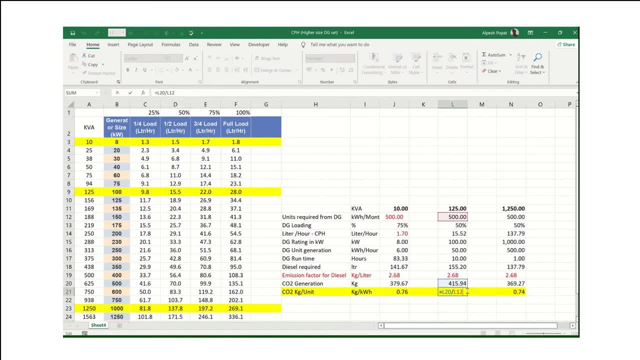 for 500. so once I divide this 500, this 4, 1, 5 divided by 500, and getting 0.83 kg per 1 unit of co2 and this one unit of co2 for one unit I have generated from 120 and then I have generated 0.5 молодdes per 1 Dragける and 1 co2 of CO2 and Routle in the. 125 kVA. Here I have generated one unit of electricity from 10 kVA DG, So here we can see that, whether it is a 10 kVA, 125 kVA or 1250 kVA, Our CO2 generation per electricity. 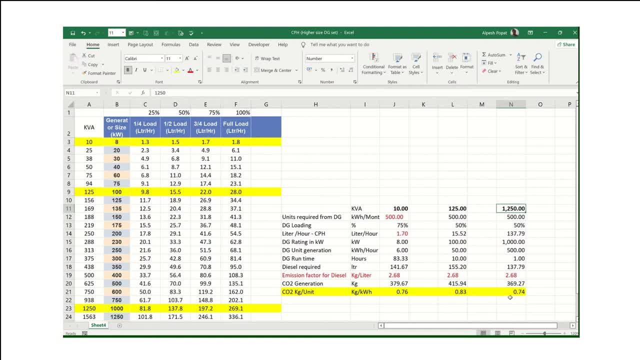 unit is 0.76 to 0.83.. It is ranging from 0.7 to 0.8.. So there is not a much difference. So we can consider the highest one, which is 0.83 in our calculation. So let us put here: 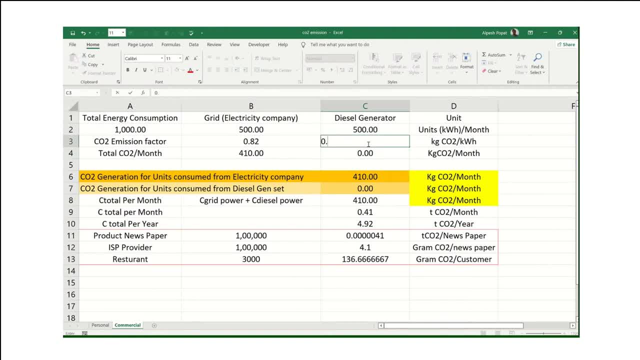 that 0.83 is my generation, So calculation is very easy for you. Here you have taken 0.82 with the power which we are buying from electricity company, and here we have taken 0.83, the power which we are generating from the diesel generator. So almost we are getting. 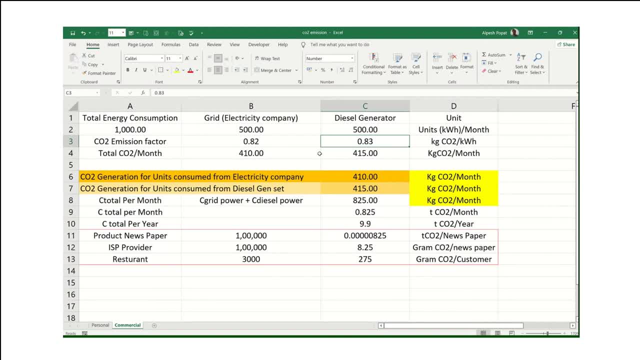 we both are same and in fact you can use it same number also just for the- you know- sake of calculation. there is no much error. So here what is the answer? CO2 generation for unit consumed from electricity company is 410.. So 410 kg CO2 per month. Similarly, 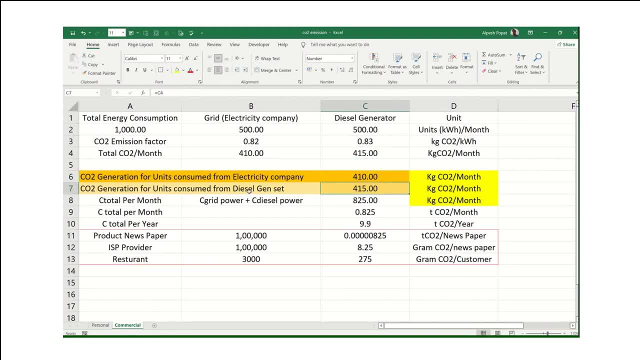 415 is a kg CO2 per month from the diesel generator. What is my formula? Total carbon dioxide generator per month is equal to C grid power plus C diesel power. That means 410 plus 410.. 415, that is becoming my total CO2 generation and that I can say ki I am generating 825. 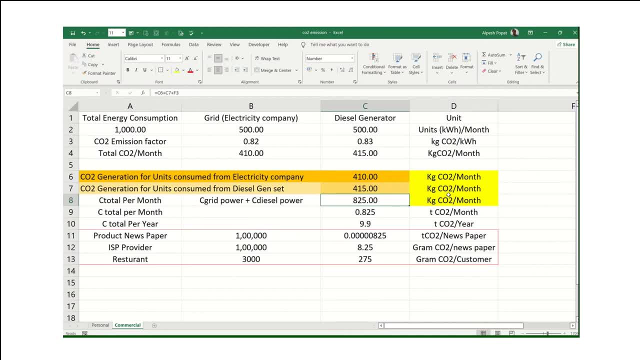 kg CO2 per month. If answer: wants in a ton of CO2, because normally these all numbers are getting reported on yearly basis. So if you want to convert this into the ton, we have to multiply by, we have to divide it by 1000. So we will get ton CO2 per month. You can. 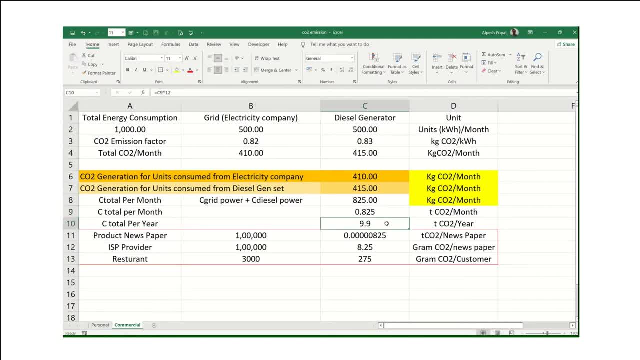 multiply by 12. So you can get annual CO2 generation of the premises. Now just for an example, once we know that, okay, I am generating 825 kg CO2 on monthly basis. Now let's say I am a newspaper company and I am using this thousand units monthly basis to run my machines and my machine. is actually producing one lakh of CO2 per month, So I am generating 825 kg CO2 per month. So you can get annual CO2 generation of the premises. Now just for an example, once we know that, okay, I am generating 825 kg CO2 per month, So you can get annual CO2 generation. of the premises. Now, just for an example. once we know that, okay, I am generating 825 kg CO2 per month, So you can get annual CO2 generation of the premises. Now just for an example. once we know that, okay, I am generating 825 kg CO2 per month, So you can get annual CO2 generation. of the premises. Now, just for an example. once we know that, okay, I am generating 825 kg CO2 per month, So you can get annual CO2 generation of the premises. Now just for an example. once we know that, okay, I am generating 825 kg CO2 per month, So you can get annual CO2 generation. 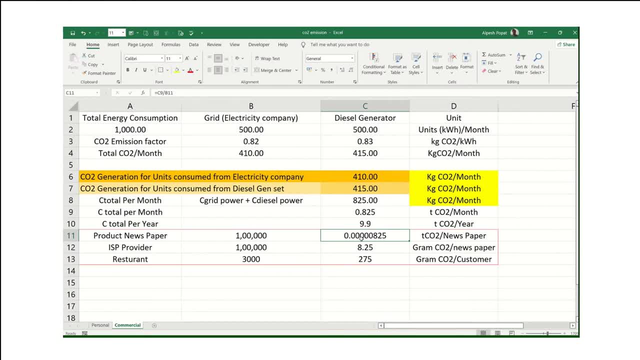 of the premises. Now, just for an example, once we know that, okay, I am generating 825 kg CO2 per month, So you can get annual CO2 generation of the premises. Now just for an example, once we are generating. so we can simply divide this 0.825 into one lakh, divided by one lakh, so we 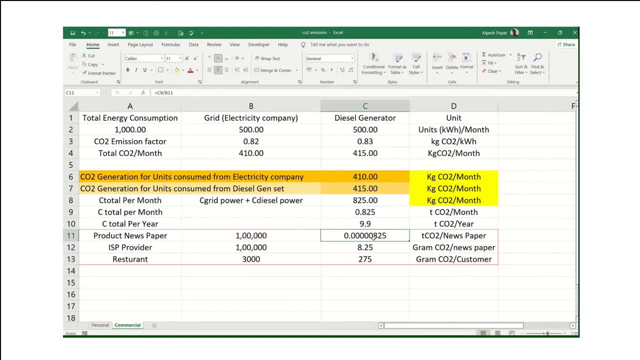 will get that for every newspaper. we are generating this much of carbon dioxide. now this is uh in a ton co2. so if you want to calculate into the kg, just to read properly, it is a 0.00825 and if you multiply further you will convert from kg to gram. so that means here we can say this is a. 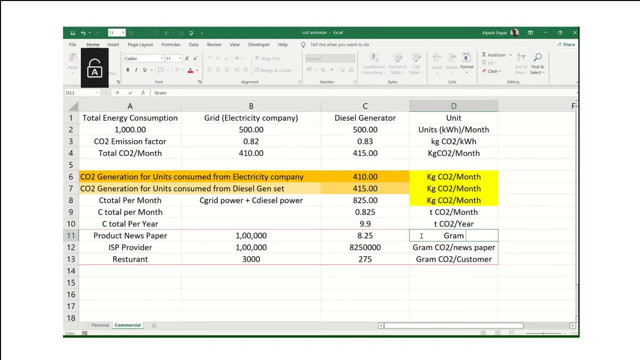 gram co2. right, this is a gram co2 per newspaper. this is how we can report. similarly, if anybody is uh like a isp provider who is providing the internet services, so let's say they may say that they have sold a hundred thousand gigabyte of data. so, simply, they can divide, you know this into, uh, this one, and they can say: 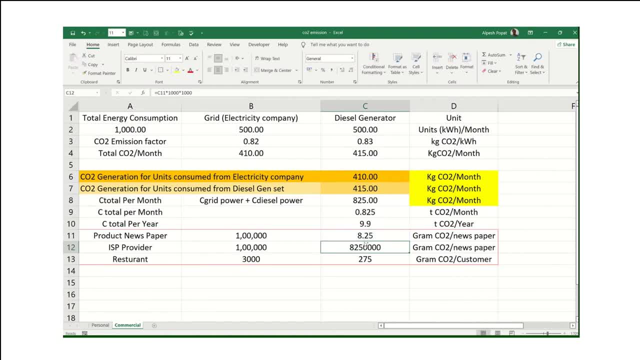 how much of uh. they have taken this here. we have changed this, so that's why it got changed. it is linked with this. okay, like that. so if we want to calculate uh from this, one number turns you to the gram co2- we have to multiply by 10, raise to 6, we will get 8.25. 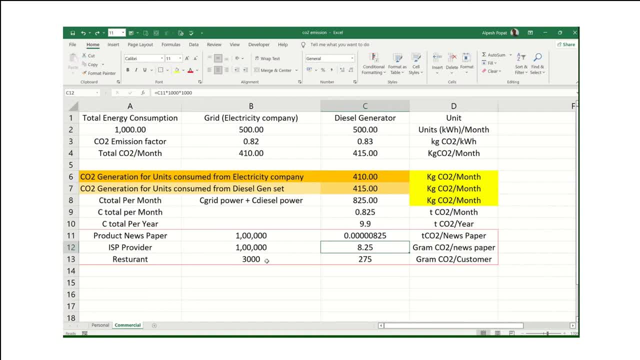 similarly, if it is a- let's say it's a restaurant, and restaurant is serving a 3000 customers every month. so what we can do. we can see that. what is my monthly co2 generation? 0.825 ton. so what we can do: we can multiply this one 0.825, divided by 3000, into 10, raised to 6, so we will get 275 grams. 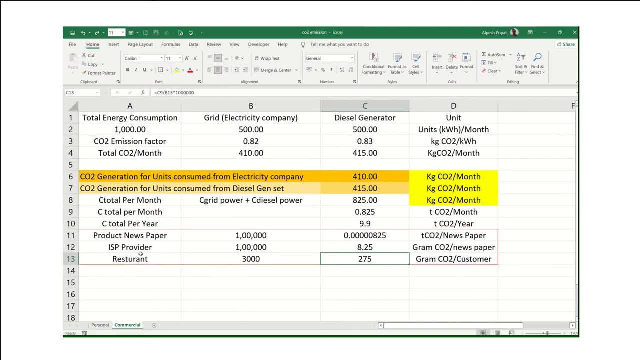 275 grams co2 per customer. so in future you will see that every restaurant, any company, any horse, any colleges, hostels, government, corporate houses, all these, they will be published their co2 numbers in form of customers or in form of month, that this is what they are generating and that's. 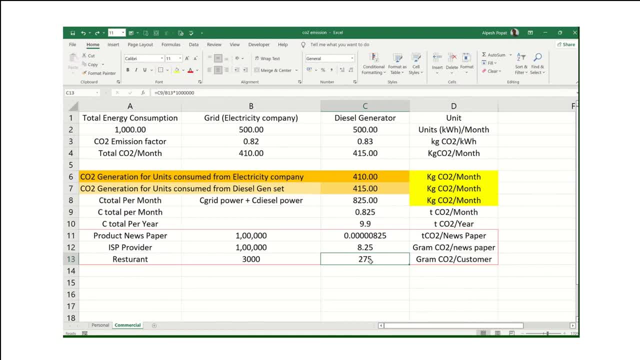 how people will come to know. for example, one restaurant is saying that they are generating 275 grams co2 per customer and if another restaurant is saying they are only generating 100 grams co2 per customer, that means that restaurant has a green power and their energy efficiency is very. 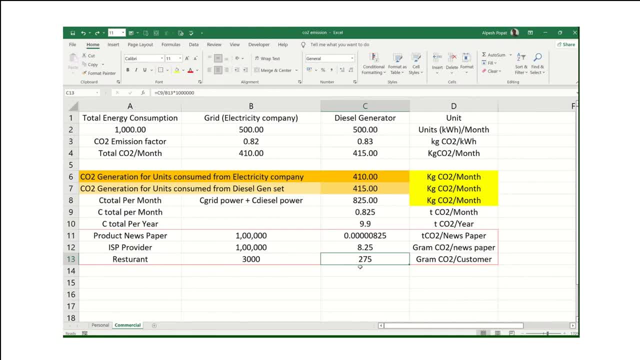 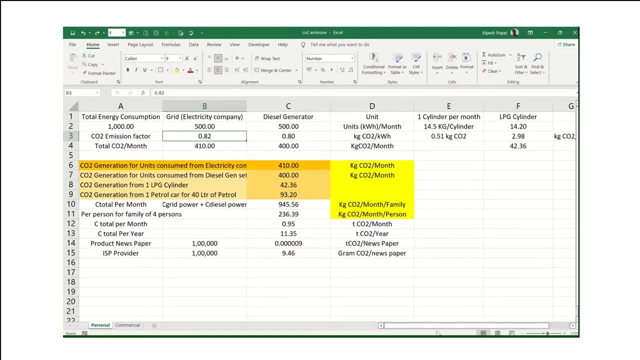 good. that's why they are contributing a less carbon dioxide into the environment and they might get some taxation benefit also. so this is the one case, what we have done for the commercial purpose. now this is the same case we can use for our personal also. let's go so in this sheet same. 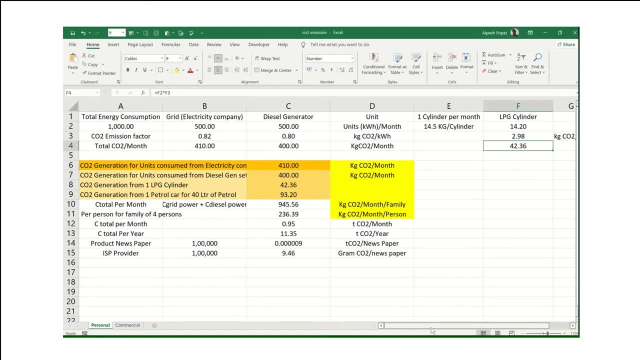 numbers i have used only. what i have added is that domestic consumption, like any family, is using a cooking gas which is lpg. so normally one cylinder of lpg is having a 14.5 kg of propane gas. okay, so if we convert this- 14.5 or 14.2, whatever- this is the emission factor for the 1 kg of gas when we burnt. in the lpg, then 2.98 kg of co2 is getting emitted into the environment of 1 kg of lpg gas. so when we burnt entire one cylinder that means 42.36. here is the calculation: 42.36 kg of co2 is emitted. 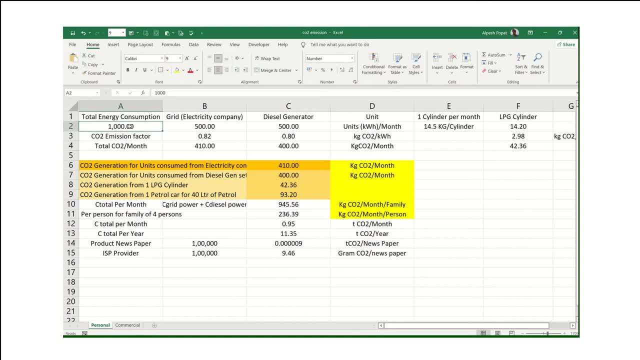 so here, if we see that same, my thousand unit is my monthly consumption: 500 from electricity board, 500 from diesel generator set, and then i will be having 810 units uh 10 and 810 kg of co2 per month for electricity. now i am adding a one cylinder as a monthly usage, so that will be add my another 42.36 kg co2. per month. and if, let's say, if i am using a petrol car and i am using a one full tank in one month, so for a one liter of petrol it will generate 2.33 kg of co2. so that's what the difference in diesel and petrol, because one liter of diesel is generating. 2.68 kg of co2, whereas one liter of petrol will generate 2.33 kg of co2. so if i convert this 40 liters, this is a 40 liter of my fuel tank, and this, if i convert this 40 liter, into. 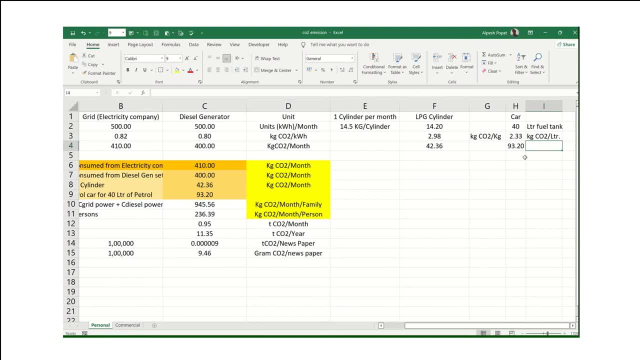 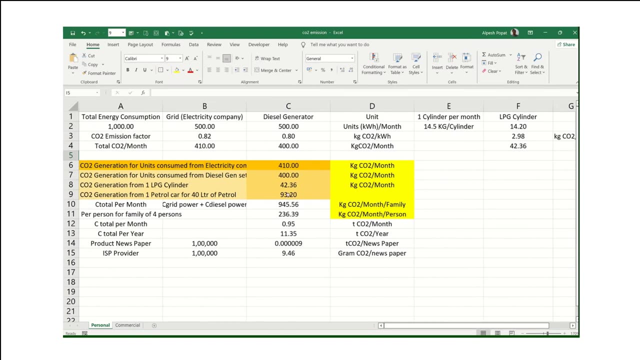 this one, so i will get 93.2 kg co2 for my fuel. okay, so this is what the liter i am burning in my driving for one month. so this is a 93.2. so if i see that, my electricity, then my cooking gas consumption and finally my uh, uh, traveling, uh, all i am adding, then it is coming. 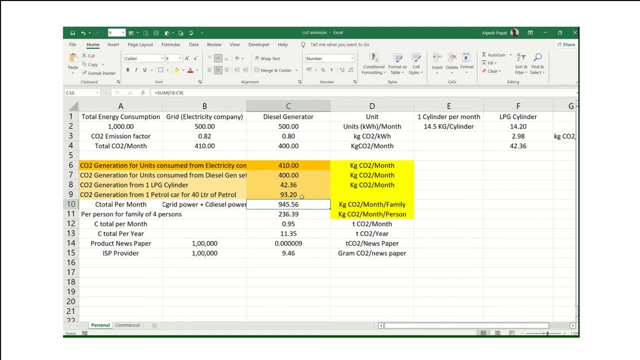 a 945, that means roughly 1000 kg. okay, so one ton of co2. uh, i am actually uh producing uh per month basis. so if i am family, so i may say 945 kg of co2 per month per family and let's say in a one family. 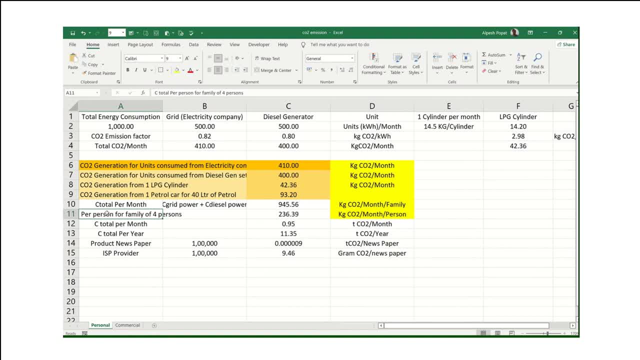 there is a four members who is actually actively using electricity- cooking and traveling. so i will divide this: 945 divided by four. okay, so then i will be saying that per person, that means i am a one person. so i will be consuming 236.39 kg of co2 per month. so this is what, uh, the calculation here. we can convert this. 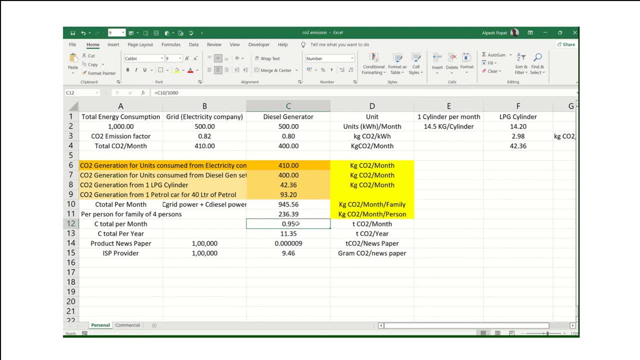 945 into a ton, so we can say 0.95 ton, which is a one ton, and if we somebody says how to calculate for one year, so you can simply multiply by 12. okay, and same thing. we can convert this co2 in some in terms of products, but anyway, product is. 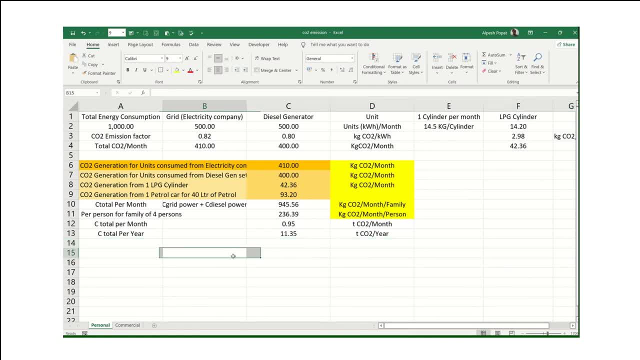 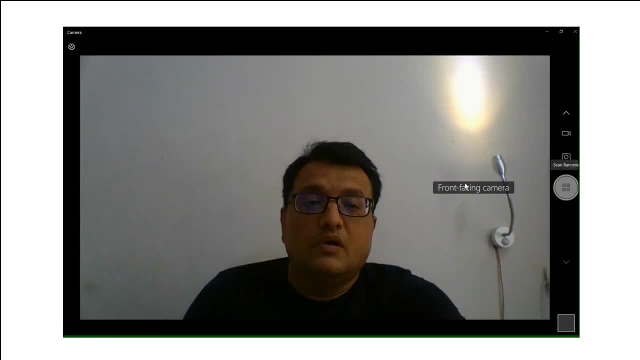 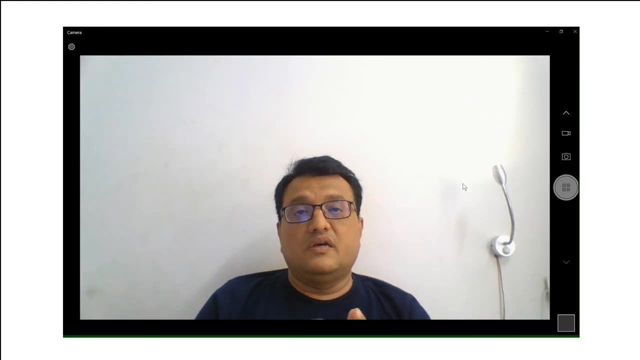 not applicable for the personal use, so we can. this is what the final calculation we can derive on. so so i think now we are pretty clear that how to calculate the co2 emissions. we have seen the guidelines also, like for grid, it is a two point. uh, it's a 0.82 kg per one unit of. electricity and for diesel generator set same number you can use, because whether you are using a 10 kva dg or 1000 kva dg, roughly your kg per unit consumption of co2 is same, which is varying between point seven to point eight two, so that is not a big difference. you can use a point eight. 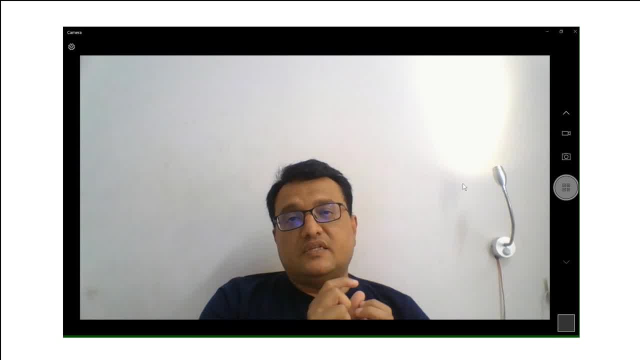 two for electricity and for diesel. electricity you can use the emission factor, point eight, two kg c o 2 per kwh. then for cooking gas we know that one kg of lpg gas will produce a 2.99 kg of co2. so that emission factor we have used. and for if i'm using a diesel car, then you can use a 2.68 liter per 2.68 kg co2 per 1 litre of diesel. and if we are using a petrol car, then we can use a 2.33 kg of co2 for one liter of petrol. so with these, 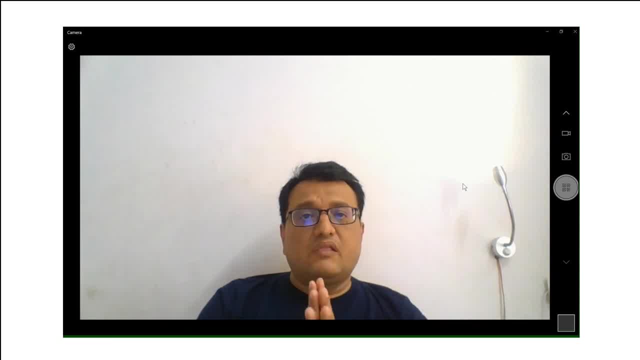 four parameters. i think you can easily calculate the your consumption. if you are using a cng gas or natural gas, then you can just go the google and you see it. then you will get emission factor for natural: one kg of natural gas or one meter cube of natural gas. what is the kg consumption? 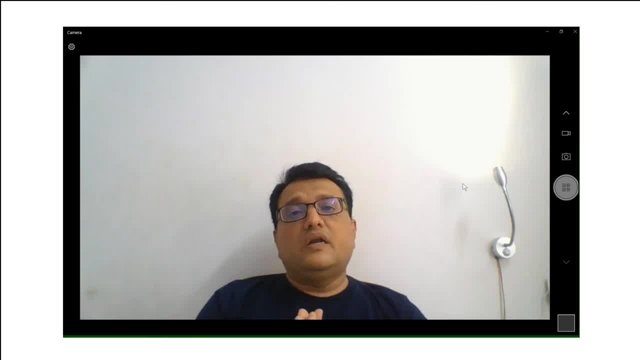 of co2, that number, you can use it and you can calculate the co2 emission and you can keep this data, you can prepare a trend and you will come to know that how your co2 consumption is going. once you know the co2 consumption, let's say, as a person i know that my family is consuming a 945. 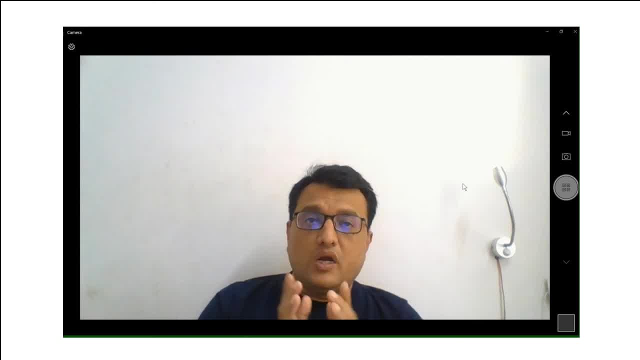 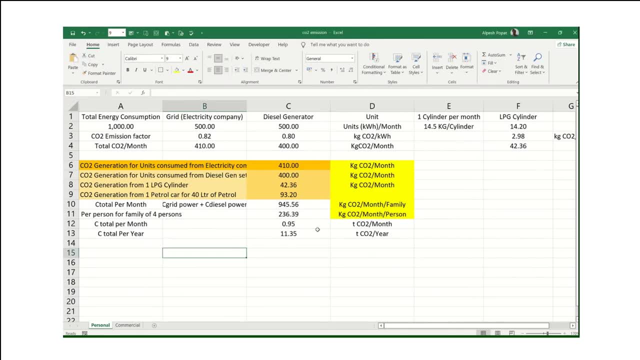 kg of co2 per month. that means almost a one ton. now, if i want to reduce my things, then i i know. if you see in this excel sheet, let's say i, somebody is giving me a target. there's this 945, which is my consumption. i want to. 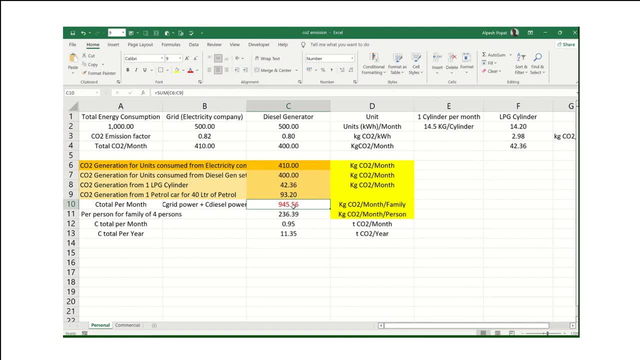 reduce by 50. okay. so when i i am saying that i want to reduce my co2 emission, so i need to see that how much co2 i am getting from you know from this. so if we say, if we let's say, divide this 4: 1. 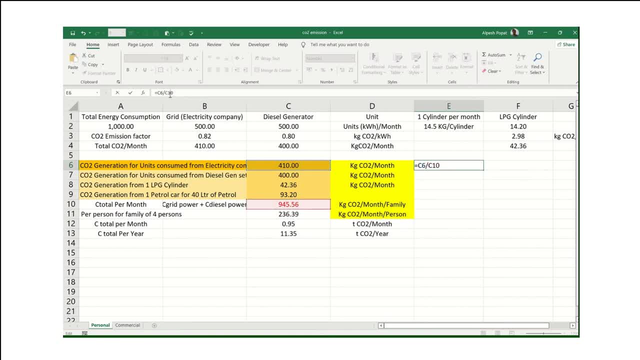 10 divided by this, and i will just freeze this number here. so we will say that, uh, we are getting 43 co2 from our electricity, which is from the electricity company, 42 from diesel generator set, then 4 from this one and 10 from the my driving. so how i can reduce what is. 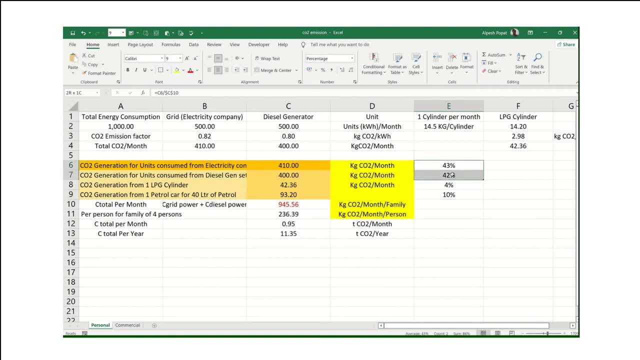 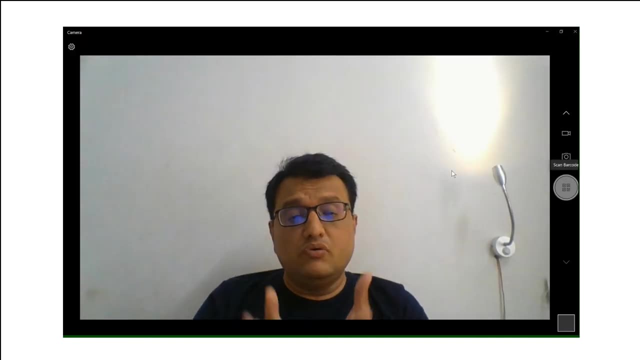 a way of reduction. so we know that these are the main two factors where highest consumption is happening, which is almost 85 percent. so if this 85 percent is coming for my electricity use, so that means i need to. what i have to do now? i have to either reduce my consumption- is it possible in today's scenario? no, we cannot reduce our. 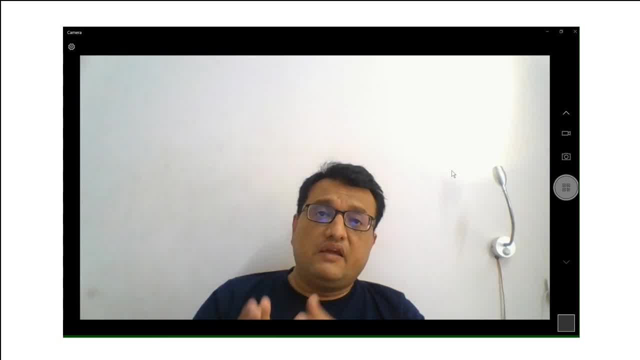 consumption. in fact, we are buying new gadgets and high fast chargers and many other things. we are keep buying. so there is no possibility that we can reduce the consumption. so consumption is going to increase. but what we can see, we can adopt the consumption and we can reduce the consumption. 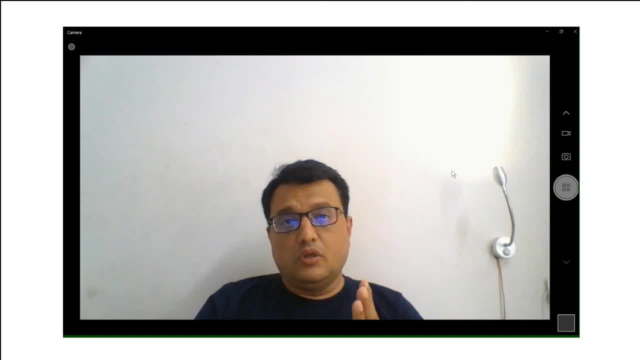 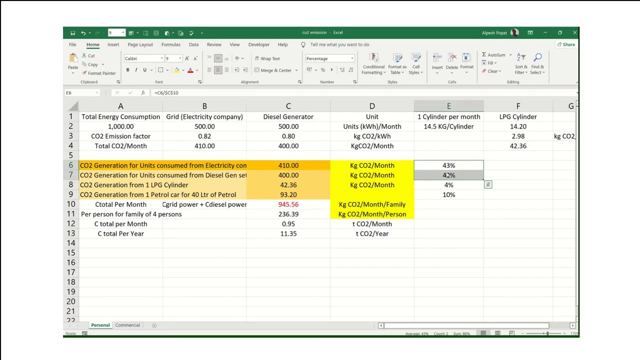 power we can do. we can buy new technologies so we can go with the solar or wind or hydrogen, whatever the technology is available in the market for the usage that only we can do. we cannot invent anything. so let's say that i need to reduce my consumption 40 by 50. so i will say that this 400. 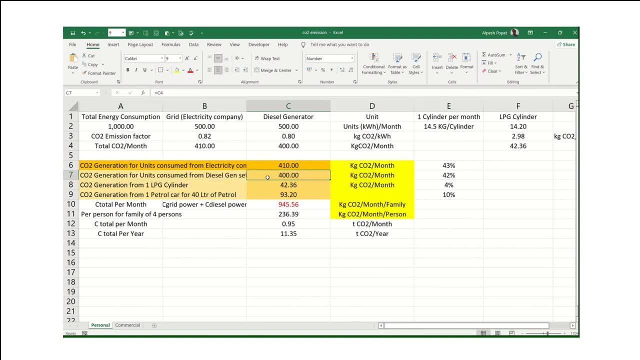 units which i am producing from the diesel generator set that i will not produce. i will remove my dg set. so this 400 units which i am producing, which i am producing from the diesel, i will not produce. i will remove my DJ set. so these 400 units which i am producing from the diesel, 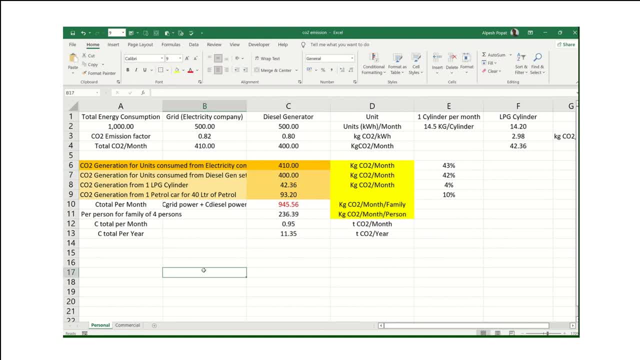 units. I want to buy from solar, for example, 400 units from solar. this is my requirement. so if you see, in my another tutorial we have given the calculation. I will simply again just mention: you can divide this: 400 divided by 3.5. 3.5 is a. 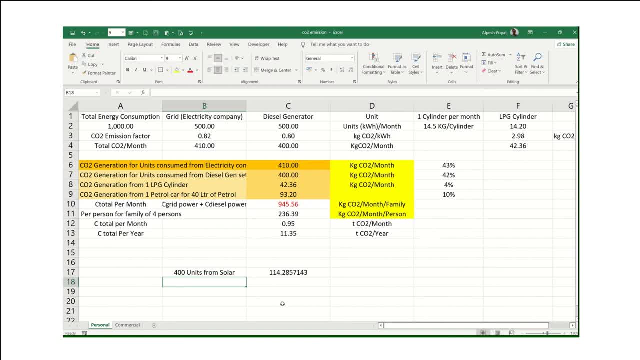 factor like 1 kilowatt of solar panel will generate a 3.5 to 4 units per day. so I'm just making some oversizing. so I am taking 3.5, so that means 400 units when you require okay from the solar. and that is for the 300 days, a 30 days. so we 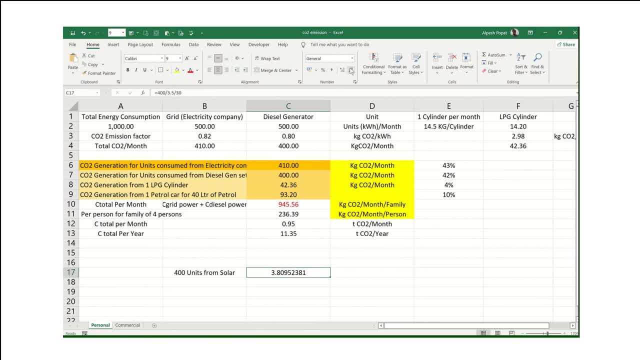 will divide by 3, so roughly we can say that we require a 3.8, 1 or 3.8 kilowatt of solar panels. I require that is the sizing of my solar panels. I require that is the sizing of my solar panels. I require that is the sizing of my. 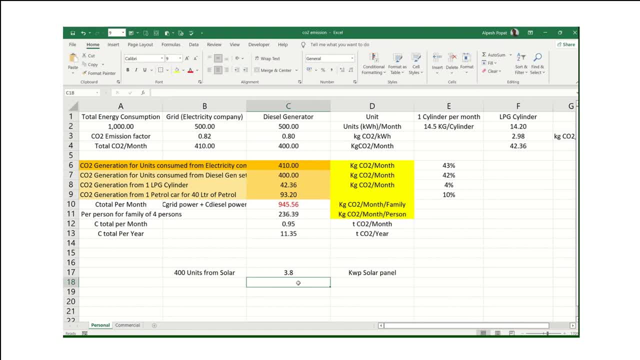 solar plant. so either three point or eight or nearly, you can go for the four kilowatt of solar panel. so once you install a four kilowatt of solar panel you will be able to generate the 400 units from the solar panel and basis you. 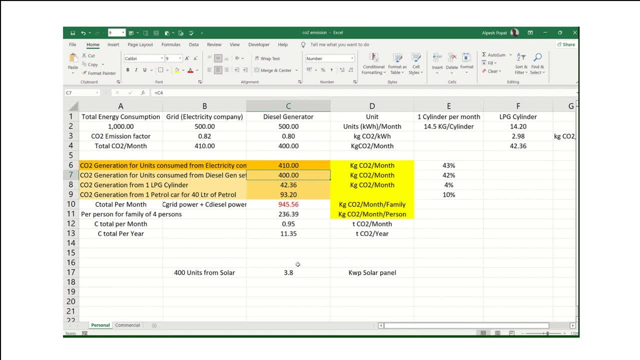 will reduce the 400 you will this 500 units you will be able to generate. let me just see: our requirement is not 400, our requirement is 500. so we require a four point. eight kilowatt of solar panel. so once we install a four point. 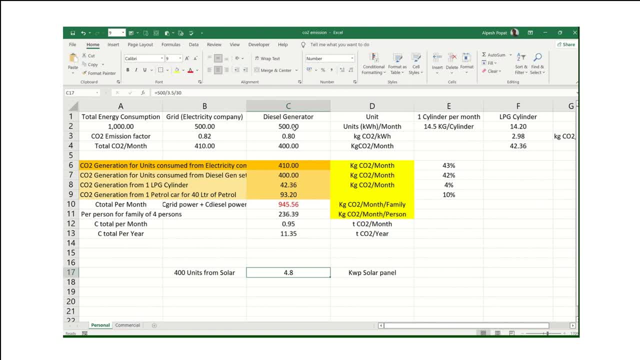 eight kilowatt of solar panel, whatever the 500 units I am getting from generator and now I am going to get from solar. so this 400 co2 emission will become a zero, because this I am now I am NOT buying from DG set and will go from. 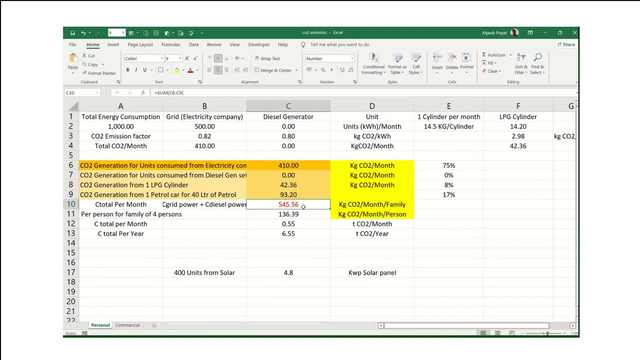 this. so now my net solar general, my co2 generation, is 545, point 56, which was earlier 945. so this is how we can reduce the our our co2 emission. so to reduce the co2 emission, what is the first thing? we should know what is my co2 emission, and then we can. 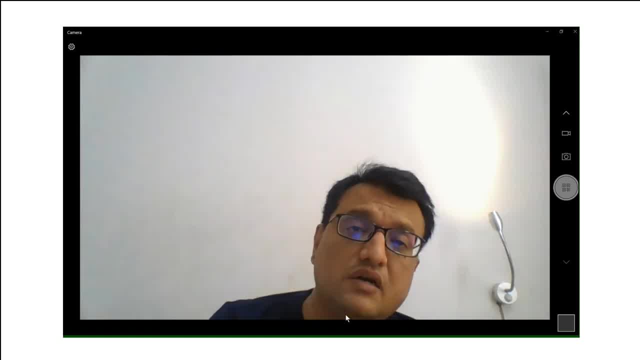 decide what, how much we want to reduce and for the reduction, what are the techniques available and basis the techniques, we can calculate what exactly I require. so with this we know we can derive the our right, you know technology and thereby we can and our choice and we can reduce our co2 generation and we can meet our target. so 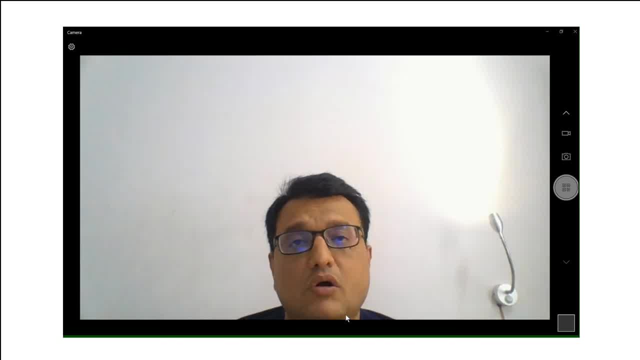 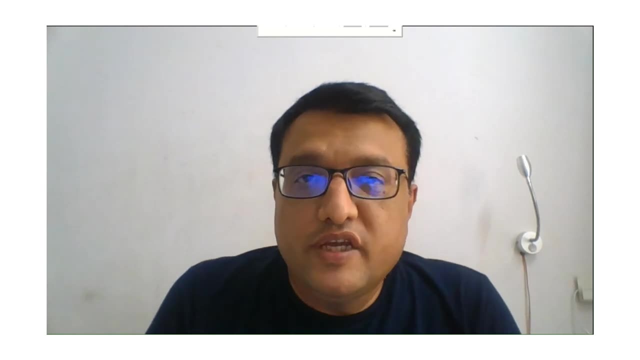 I think that this precisely. we have discussed all the topics and it will be very helpful to you, so I request that you you implement this, whatever the learnings you have got today, in your daily usage, thank you. so if you enjoy today's tutorial, please consider to subscribe this channel and hit the like.